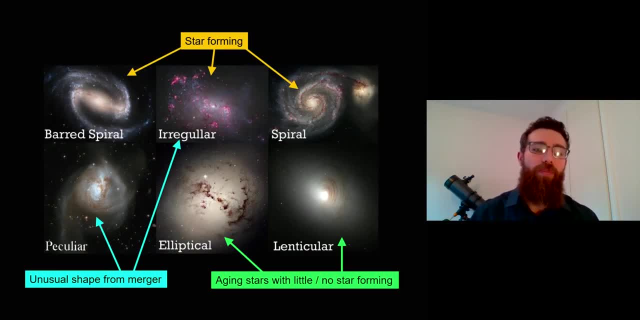 more kind of spherical looking central core or bulge. You then have the elliptical galaxies, Irregular ones. These are formed when you have galaxies interacting, So these may be from galaxies that are colliding or merging, and they have very irregular shapes, hence their name. 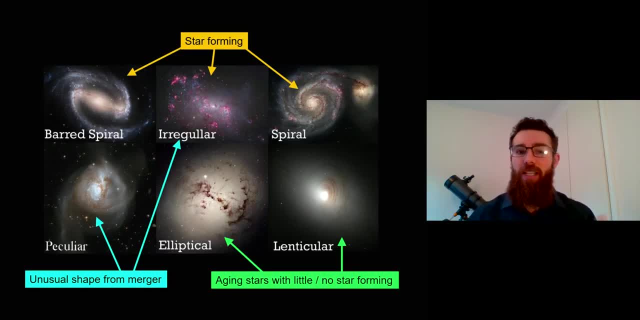 Some of them are undergoing large amounts of star formation because the gas gets compressed and it forces stars to form. And then you have the ellipticals. So the ellipticals have very little gas. They are featureless, They don't have those spiral arms, So they are basically elliptical. 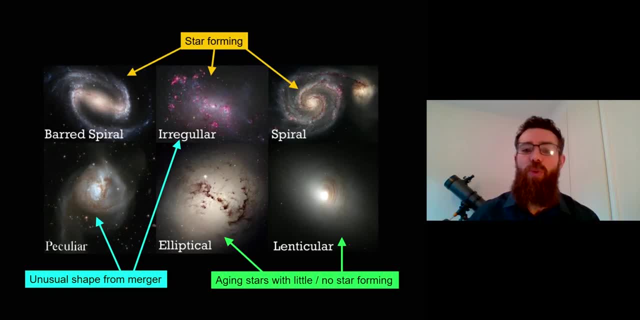 That's how they look. And then you have lenticular, which are in between the spirals and ellipticals. They have features that correspond to both. They kind of sit in between. The ones we're interested in just for this short video is the spirals and the ellipticals, and what are the main differences? 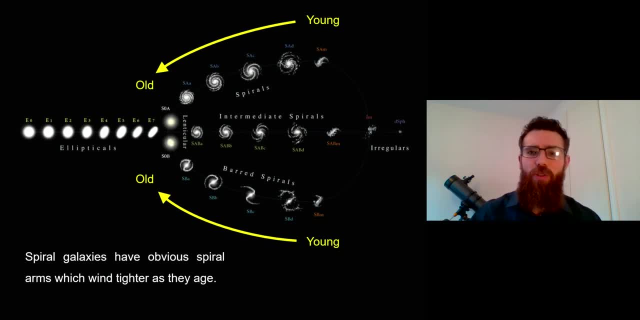 between the two. So if we go to the galaxy tuning fork diagram, which shows the different types and classifications of galaxies, it's also quite useful for looking at the evolution as well. So on the right hand side of the tuning fork you have your spiral galaxies And, depending if it's 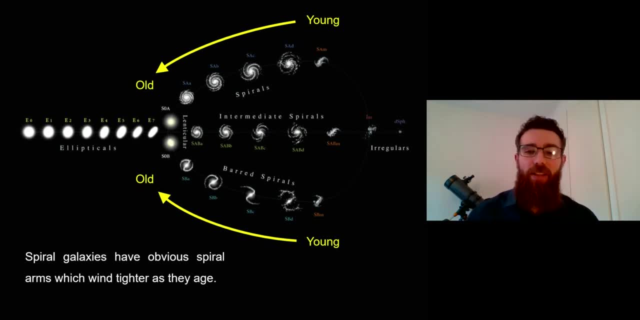 a normal spiral, a barred spiral, intermediate. that's where the different paths come from, the different parts of the fork. So what happens here is they actually evolve from the right to the left. So the younger ones are right on the right hand side and your old spiral galaxies. 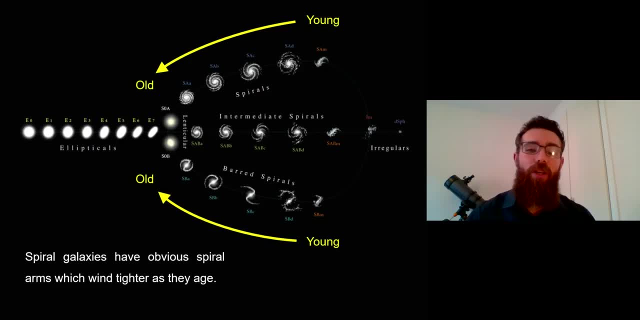 are more towards the center, across to the left of the spiral path, And it should be fairly obvious. really, they have spiral arms. That's what makes them stand out, That's why they're called spiral galaxies. But also, as they age, these spiral arms become more tightly wound. So as they age, 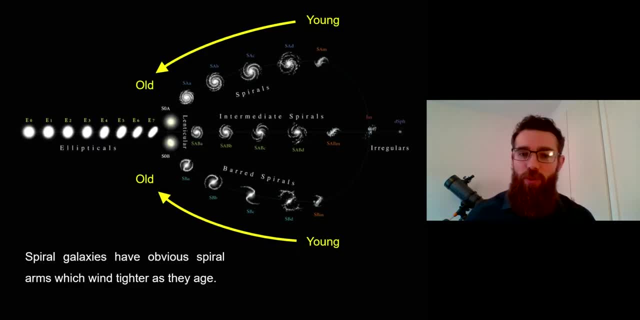 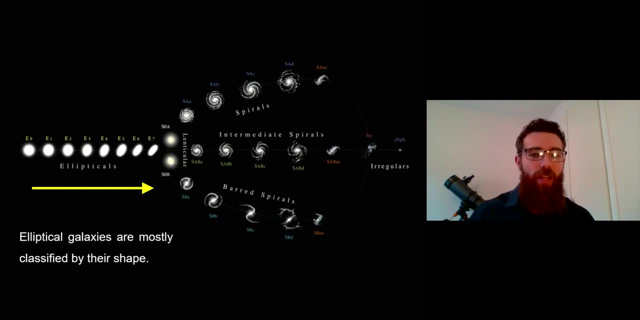 these spiral arms get tighter And a few other things happen as well. So as they go from right to left on this diagram, you'll note that they actually get a bit tighter. Now the ellipticals which sit on the left hand side of this diagram. they're mostly classified by their shape. 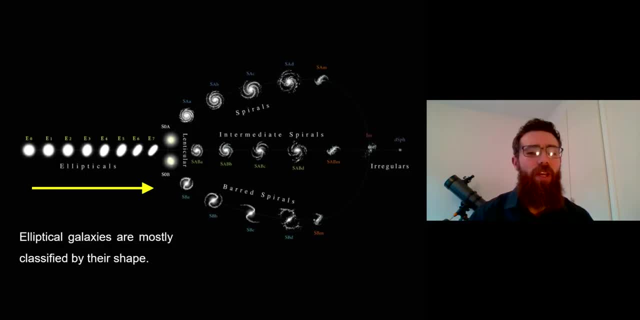 So they can go from circular to more of like a cigar shape And depending on where they sit on that scale, they'll be given some kind of number And that's pretty much the main classification for them. That's how we give ellipticals a number or a type. I suppose It's just purely on their shape, But that could. 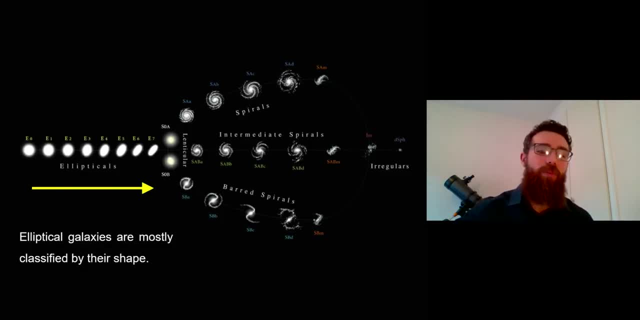 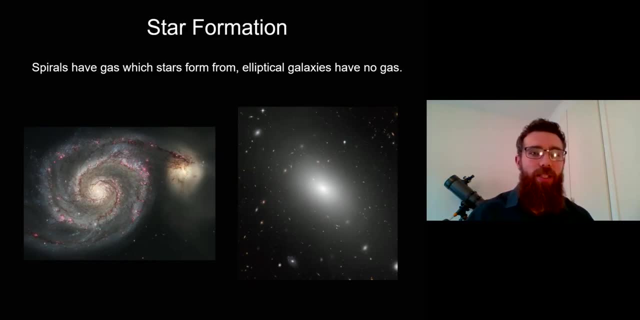 relate to how we're looking at them, the orientation as we see them when we look out into space. So one of the key differences between elliptical galaxies and spiral galaxies is star formation. So spiral galaxies: they're the galaxies that got all that gas in The gas. 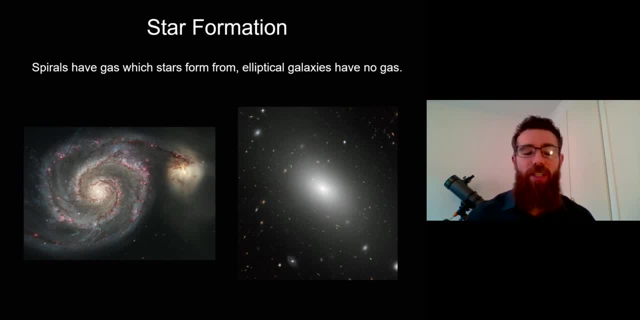 will collapse and form stars. So what you typically find is that in the spiral galaxies you've got large amounts of star formation. Now, in contrast, elliptical galaxies don't have gas in them, or very, very little, So therefore they don't have any star formation. So spiral galaxies undergoing star formation. 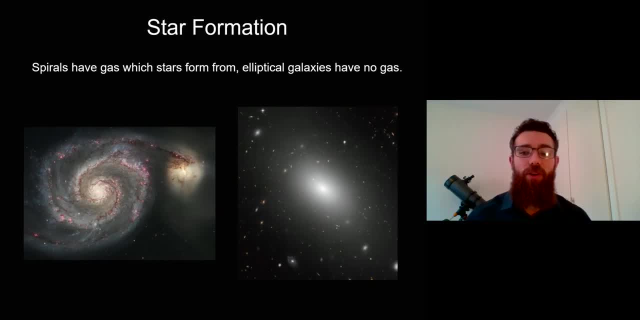 have younger stars in because they're still currently forming stars. Elliptical galaxies have older stars and they don't have those new stars that have recently been formed. So they don't have that gas. It's down to their gas content, basically, as to why one is forming stars. 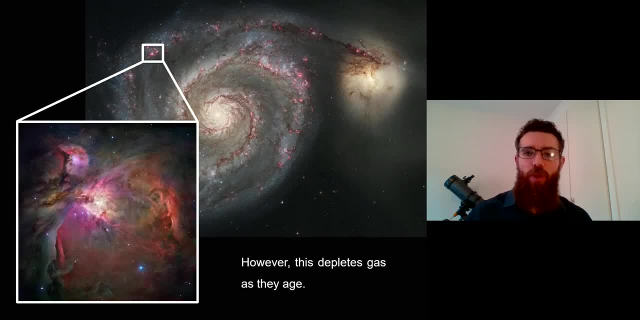 and one isn't. If we look a bit closer at a spiral galaxy, then we can see some of these regions where the stars are actually forming. So this is the Orion Nebula, which is in the white box, And you can see this with a fairly small telescope, actually yourself- And within that nebula. 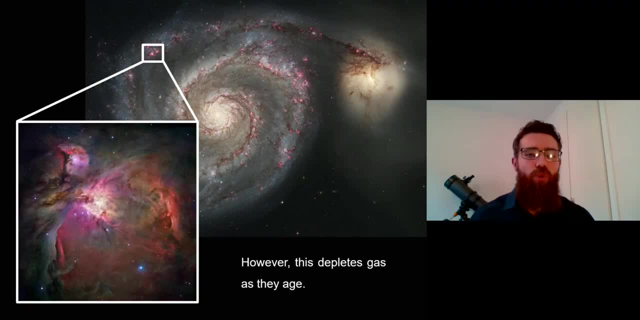 which is a cloud of ionized gas. you've got bright blue stars And it's the bright blue stars that are illuminating the nebula And if you zoom out and look at the overall galaxy, you can see that you've got. you can see regions of blue, kind of red purple. They're those areas of star formation. 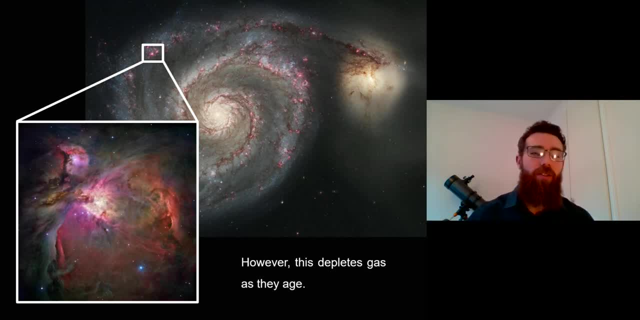 because these bright blue stars are then, you know, illuminating these clouds of gas, that they sit in these nebulas, And we can see that in the galaxy themselves. So we see these bright regions of star formation Also, as the galaxy ages, that gas. 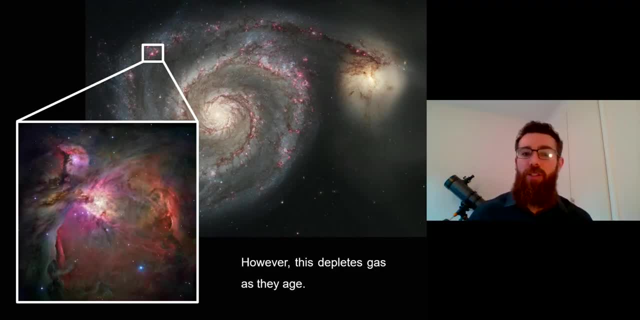 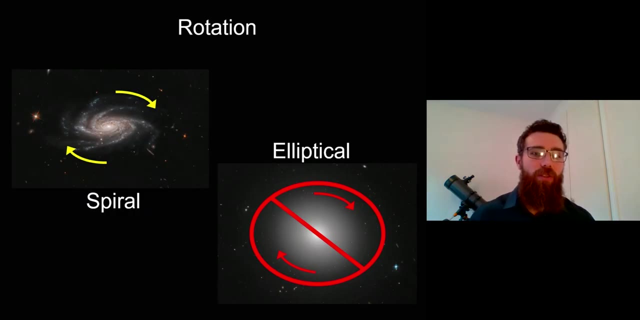 will be depleted, So over time that gas gets turned into stars and you have less and less gas in the galaxy. So therefore star formation kind of falls off as they start to age. Another key aspect between the two will probably be is rotation. So spiral galaxies would typically have some kind of net rotation. 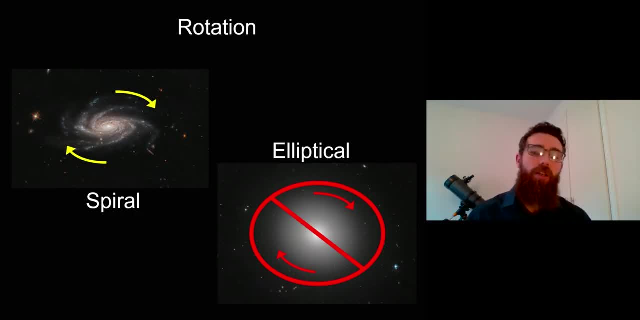 They're rotating about a centre, a bit like a disc. Elliptical galaxies don't necessarily show that There isn't always a net rotation there. The stars are moving a little bit more randomly, So dynamically. there's differences between the two. They look different, but they're also not behaving the same way. 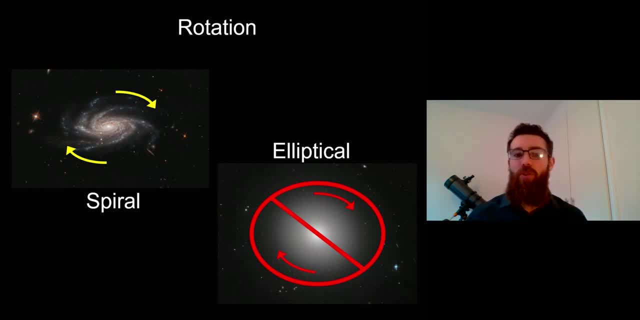 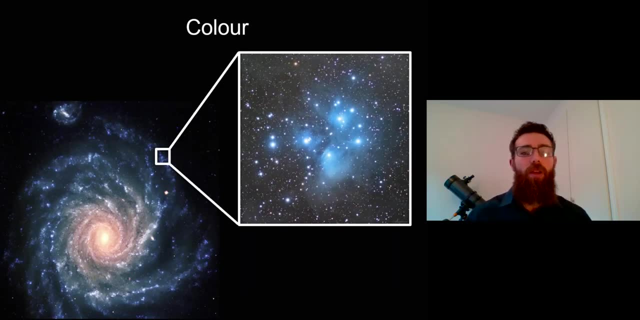 So one typically rotates in a common direction, or a bit like a disc, and the other does not, And then we have colour. So the spiral galaxies, because they have these younger blue stars, they have more of them in their galaxy, the galaxy as a 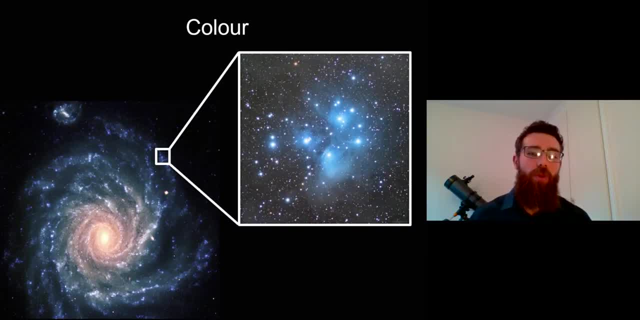 whole is typically bluer. So here we've got a nice galaxy. you can see lots of blue in it and we've got the Pleiades there. You can see the Pleiades there, Which is a cluster of very young stars You can see. they're visually blue and we'd 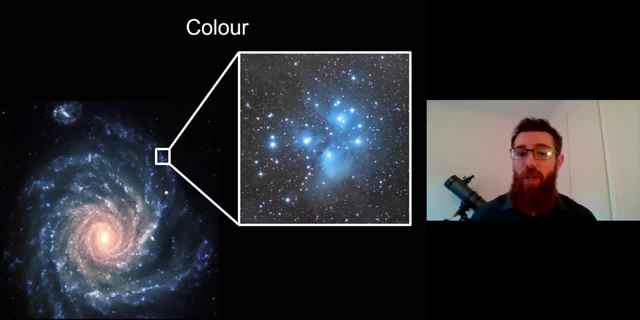 expect to find a lot of those in the spiral arms of a spiral galaxy, because that's where the stars typically form, And if there's plenty of gas there, then we're going to get lots of stars forming, So young stars are going to be bluer. 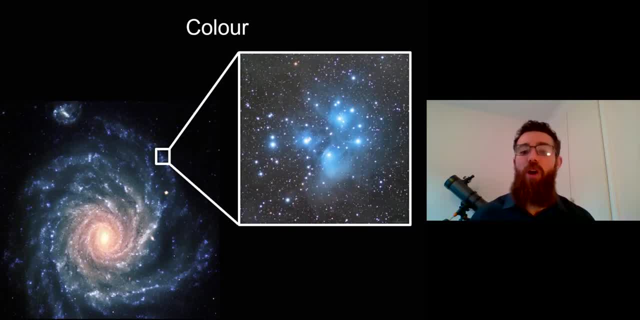 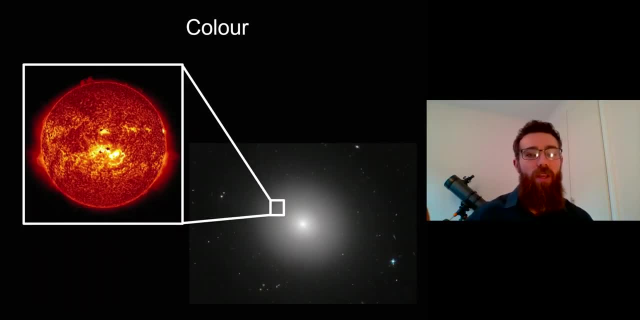 older stars are going to be redder, So we would find that a spiral galaxy is likely to be bluer than an elliptical galaxy And obviously, in contrast, we have elliptical galaxies. they don't have those bright regions of star formation And, because they haven't had any recent star formation occurring, there's 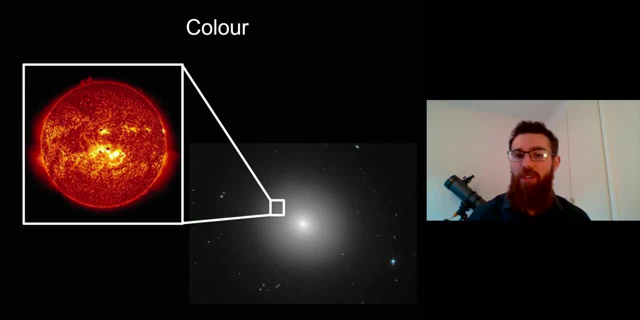 no young stars there, So it's a collection of old population stars, So these stars are typically redder. As stars age, they will get redder, And that means that if you have a population of stars that all do the same thing getting older, then the whole galaxy. 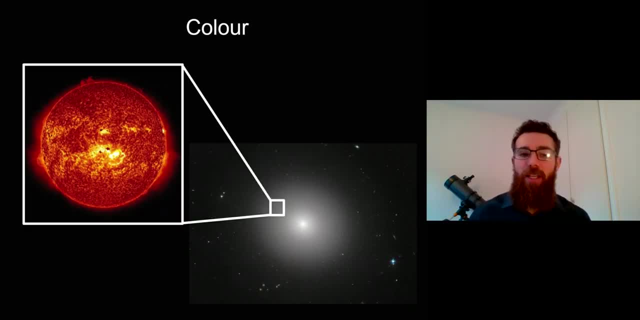 is going to be redder. So what we find is that as galaxies age, they move from being blue to red, Not exactly blue or red, but they are bluer or redder than one another. So we find that elliptical galaxies are redder because they have these older stars in them.